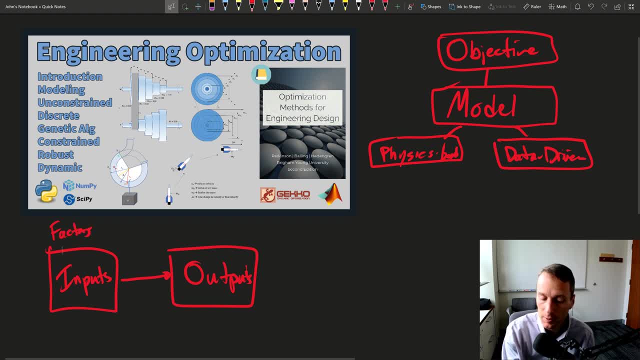 these can- okay, we call them factors, parameters or features- how they influence an outcome And in optimization we need to create this model so we can actually go in reverse. So we can go this way where we say we want to maximize or minimize something from an output or achieve a. 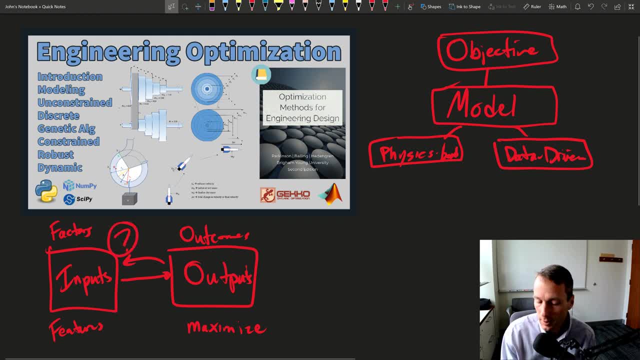 certain target. What are the inputs that are needed in order to achieve that? So, after we've created the model, we need to then do another thing, which is then create the algorithm that can then optimize this model or this process. Okay, so the next thing we need to do, 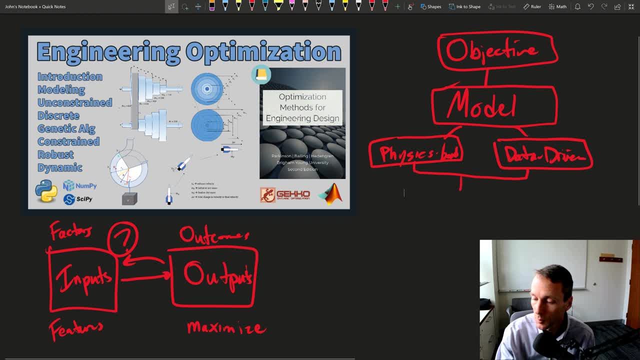 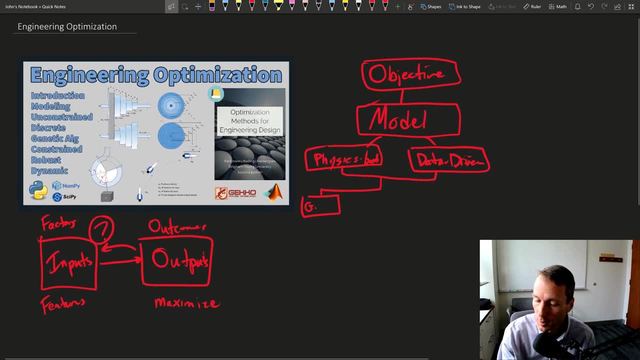 is: take these two models and we can either go with a gradient-based approach or a gradient-free approach. Okay, so the gradient-based approach. we're going to have a number of methods that we're going to use for that. We're going to first of all, explore unconstrained 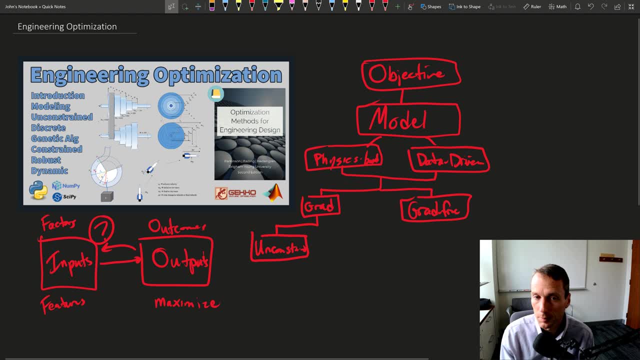 Okay, unconstrained optimization and also discrete, where some of these variables are going to have, you know, continuous or integer or discrete values. So that really comes up here with the model I'm going to write discrete type variables. Okay, we're going to talk about some. 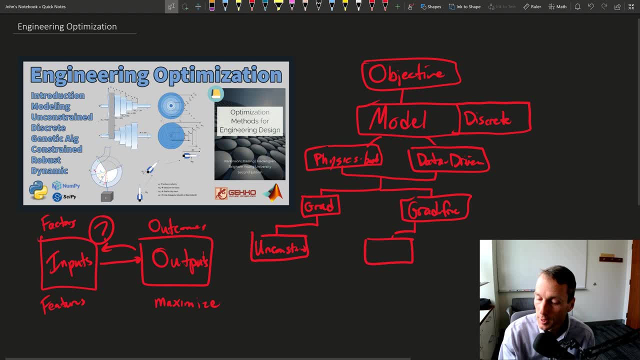 gradient-free algorithms as well, such as genetic-free algorithms or genetic-free algorithms or genetic algorithms or simulated annealing among two of those. Okay, and then we're going to talk about constrained optimization. So the KKT conditions and others that relate to how you 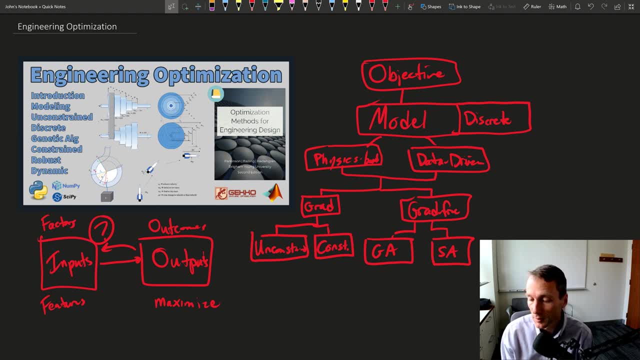 constrain some of the decision variables or even the outputs and the algorithms that can efficiently solve those with gradient-based methods, Then we're going to talk about robust optimization. So this gets back to the model where we have uncertainty And we need to be able. 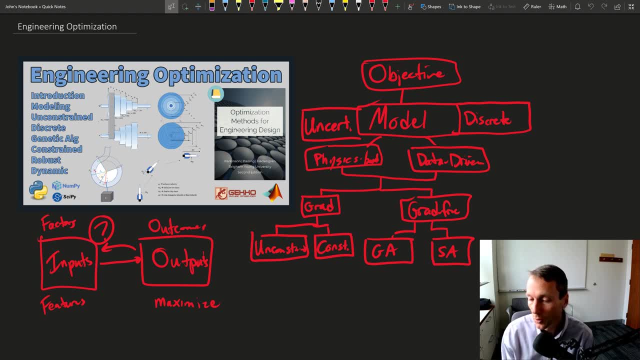 to adapt our optimization methods so that we can properly handle the uncertainty and design in safety. And you know, considering that most systems have some uncertainty in the parameters, they're not exact representations of our process And the cost of violating certain constraints is very high, So we need to build in robust solutions. 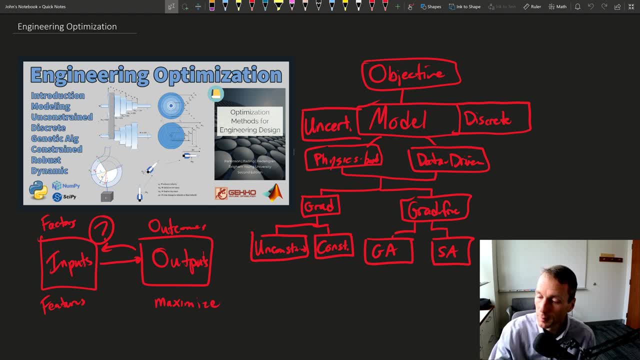 to be able to handle some of that uncertainty. And then the final one that we're going to deal with is dynamics. Okay, so what happens when the model is not static but it has some dynamics associated with it? How do we deal with that? Okay, so a lot of the course is on either the modeling or the 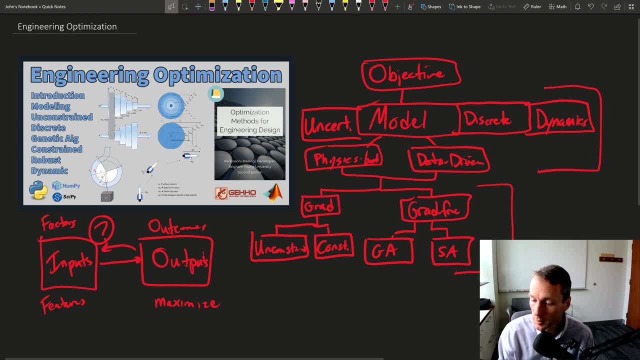 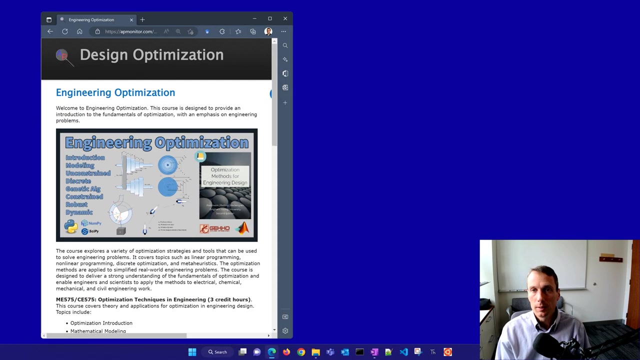 algorithm's themselves To be able to solve these optimization problems. The top part is going here, That's the modeling, And the optimization is often trying to maximize an output by changing the inputs. me give you just an overview of the course and i'll bring this over. this is the course website. 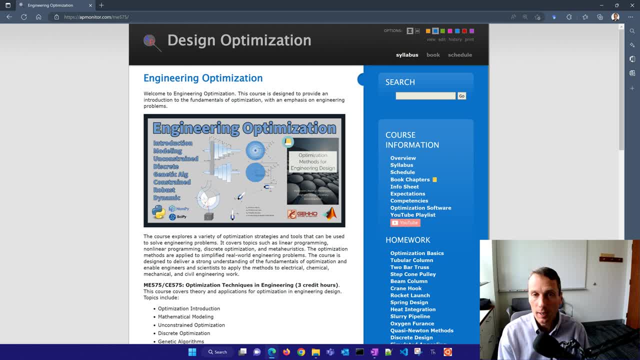 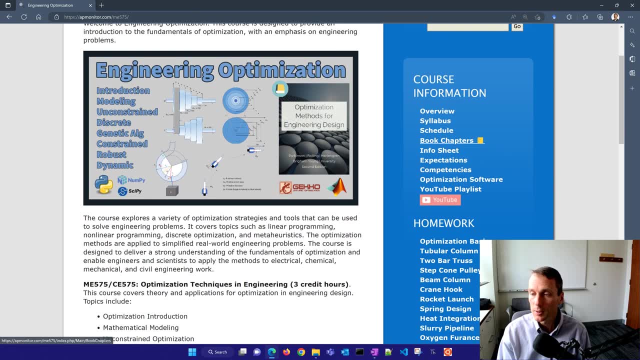 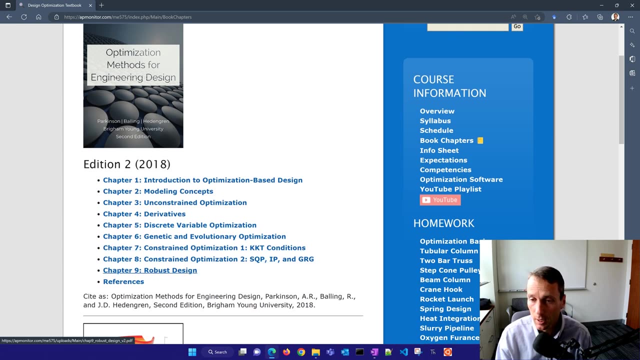 just come here to me 575, ap monitorcom, me 575, and you'll see the course and you'll see the layout here. the first thing you want to look at are some of the book chapters and you know, just go through. this material gives a lot more detail about the algorithms. there are also a number of homework. 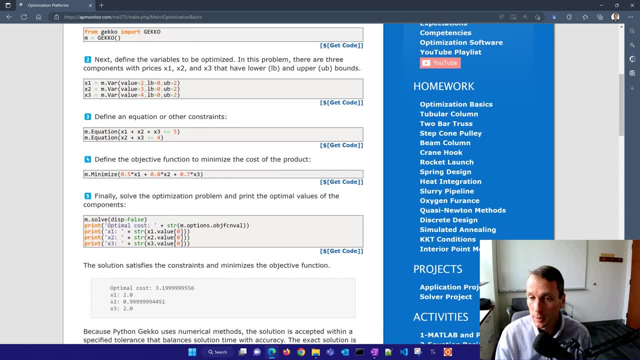 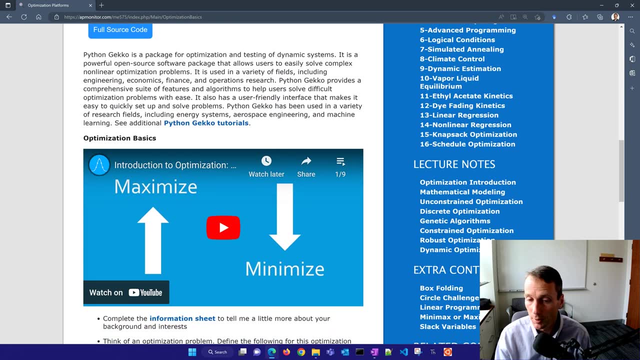 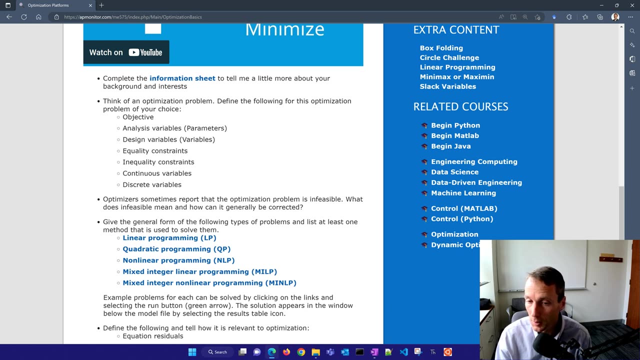 problems so you can start off with optimization basics. introduces you to python. gecko. gives some introduction to maximizing or minimizing, how you solve optimization problems and constraints. equality and inequality constraints, continuous and discrete variables. and then the different types of optimization that you can perform, like linear programming. 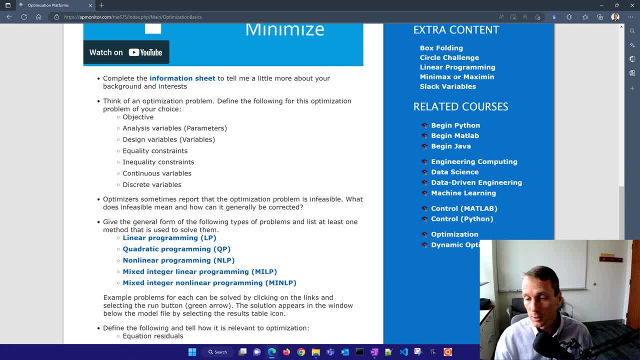 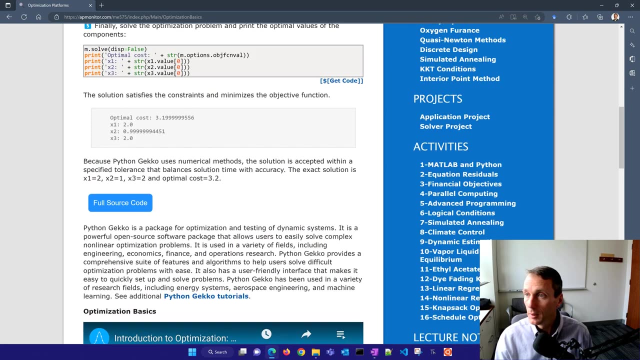 quadratic, non-linear, mixed integer, mixed integer, non-linear programming. so it gives just an overview of some of the terminology that we're going to be using as we describe these types of problems. all right now, we also have activities here as well, in addition to the homework problems.